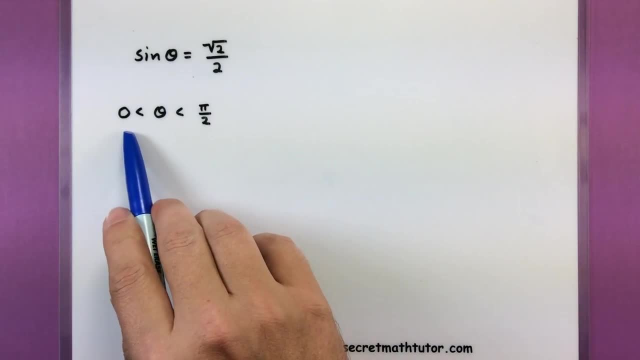 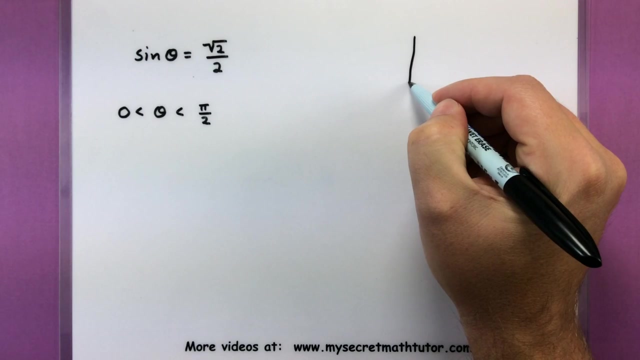 For this one I'm curious what the angle is. it lives between 0 and pi over 2, and I know that the sine of that angle is square root of 2 over 2.. To solve something like this, it's probably a good idea to just sketch out where that angle lives. So this one is in the first quadrant. 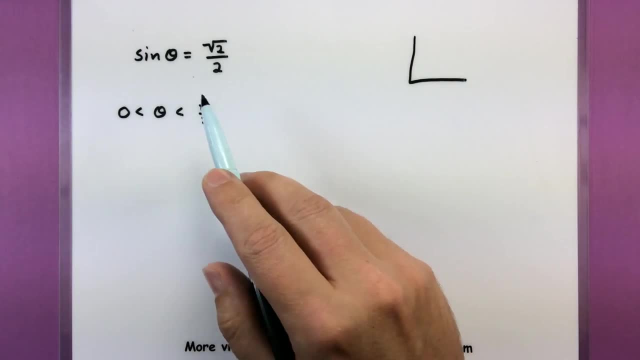 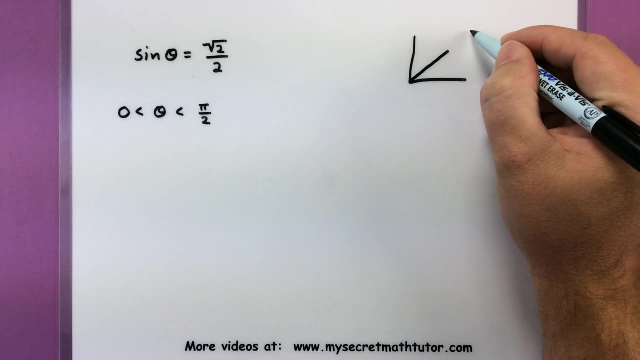 so you can imagine just looking at that first quadrant For sine. I'm thinking of my unit circle and thinking where the second coordinate is equal to square root of 2 over 2.. In my head I'm thinking of a picture like this: second coordinate, square root of 2 over 2.. 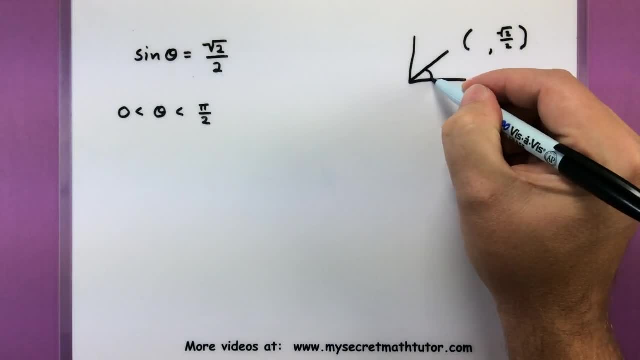 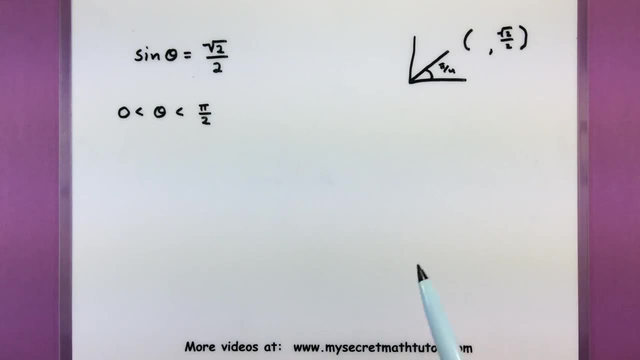 Once I have that information I can look it up and say: I remember this angle. it's actually just pi over 4.. That's the only one in the first quadrant whose second coordinate is the square root of 2 over 2.. So theta equals pi over 4, not bad. 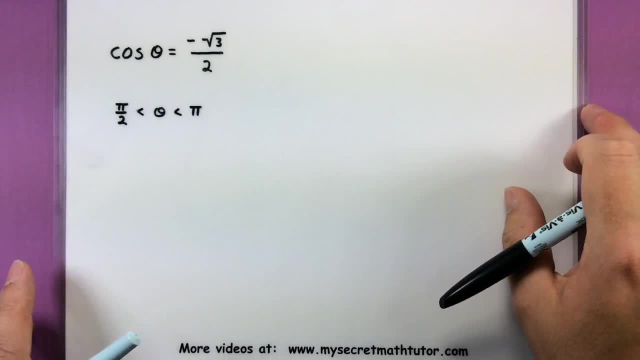 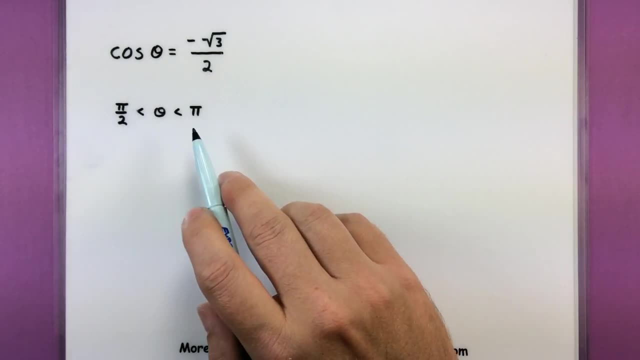 Let's try another one of these. This one says: cosine of theta is equal to- square root of 3 over 2, and now our angle lives somewhere between pi over 2 and pi. So once again, let's go ahead and just sketch out where this angle lives. 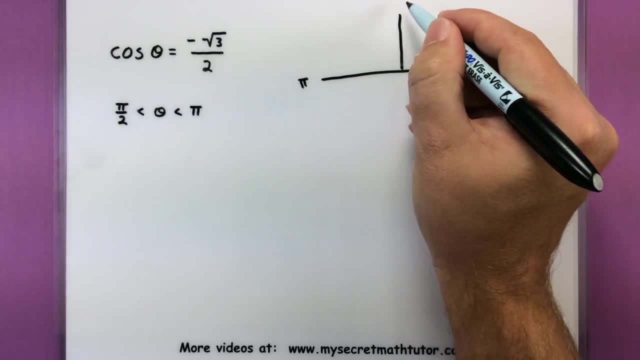 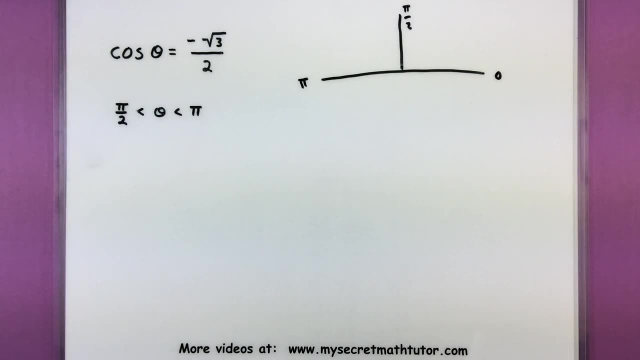 So this would be 0 degrees. this would be pi and pi over 2.. So if it's between pi over 2 and pi, we're dealing with the second quadrant over on this side. Now again, I want to think: well, if it lives in the second quadrant, what value should 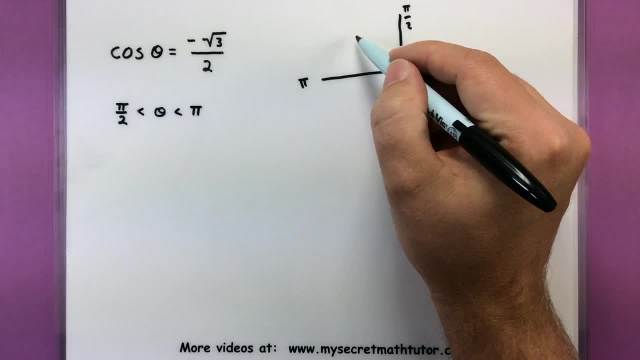 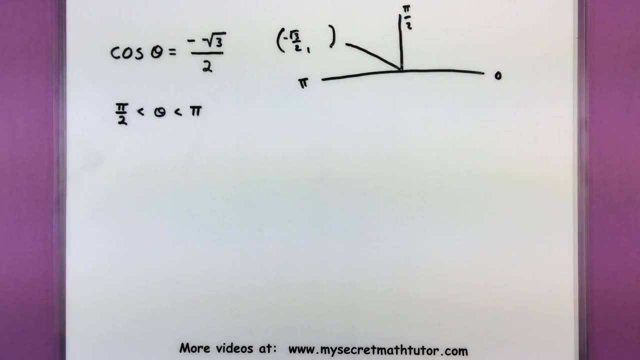 it have. We want the first coordinate to be negative square root of 3 over 2.. So I'm looking at angles. first coordinate has to be negative square root of 3 over 2, and now I just have to figure out what that angle is. There's a couple of ways. 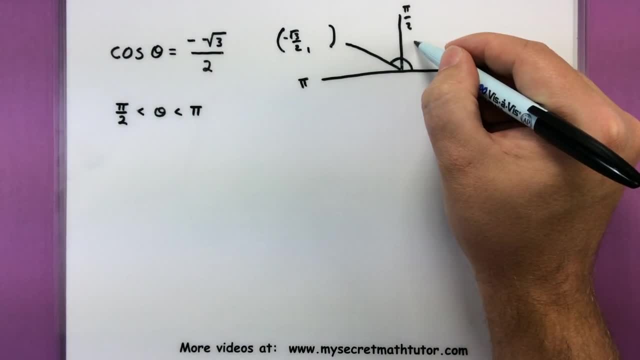 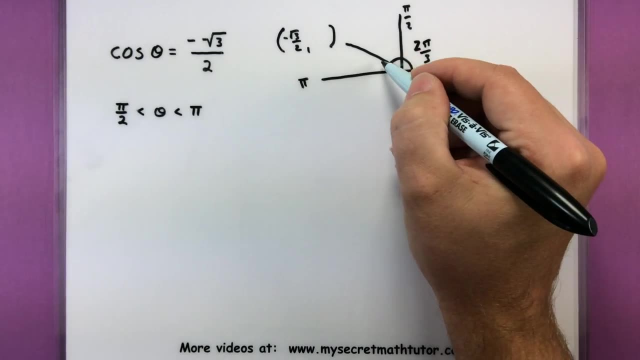 you could do it. If you actually just look it up in the unit circle, you'll find that it's at 2 pi over 3.. If you're only looking at the first quadrant, then you want to think of reference angles that have a reference of pi over 3.. And 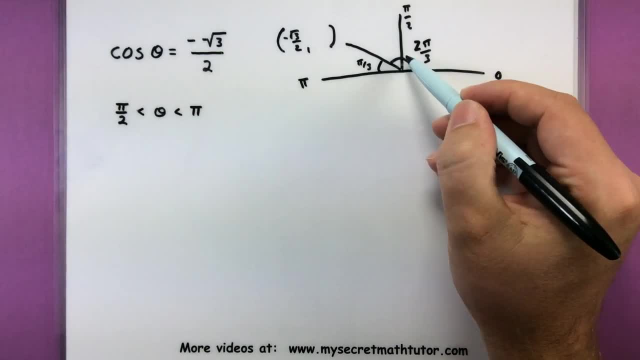 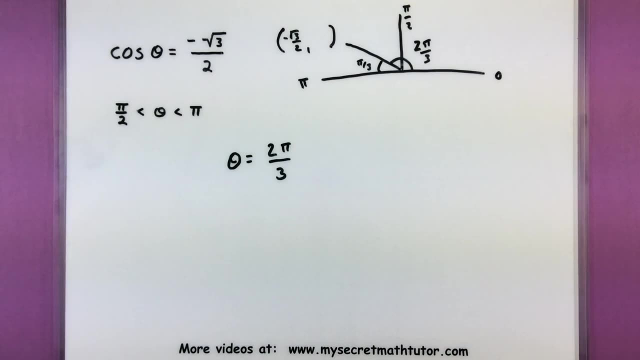 of course, make sure your signs match up. Anyway, this one is at 2 pi over 3, so sure enough, that is our angle: 2 pi all over 3.. Now, sometimes you might come across problems where more than one angle will satisfy the given conditions, And if that's the case, you really just 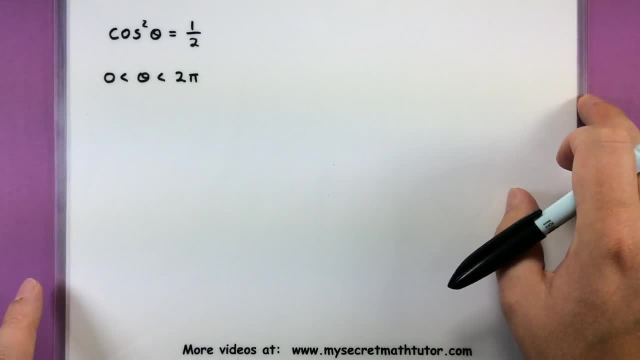 want to list out all the angles that work. Let's try this one. This one: my angle could be anywhere in the circle, anywhere between 0 and 2 pi, And what I know about it is that if I square cosine, I get a value of one-half. 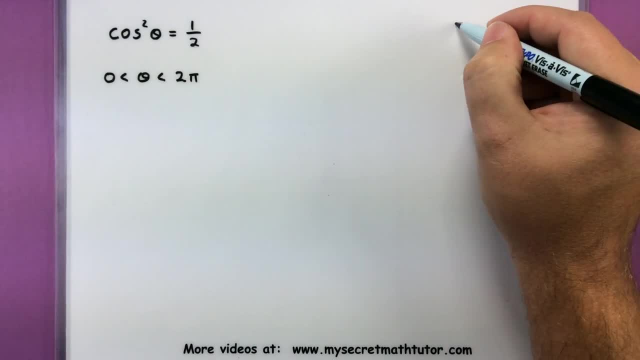 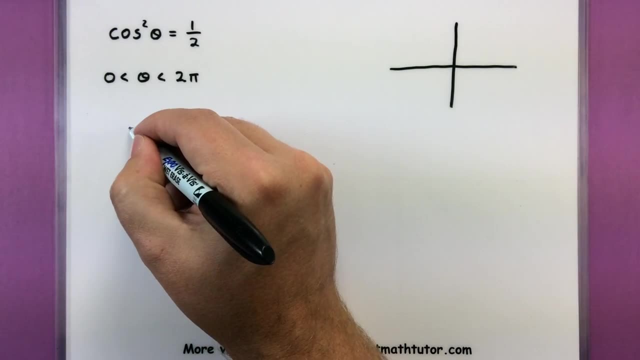 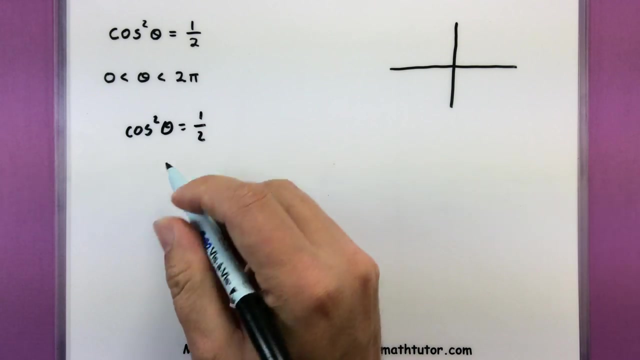 So we're going to have to work with this a little bit and, of course, really think about all the values that show up as we go all the way around that circle. So one-half is one of my key values that I'd be looking for on my unit circle. but 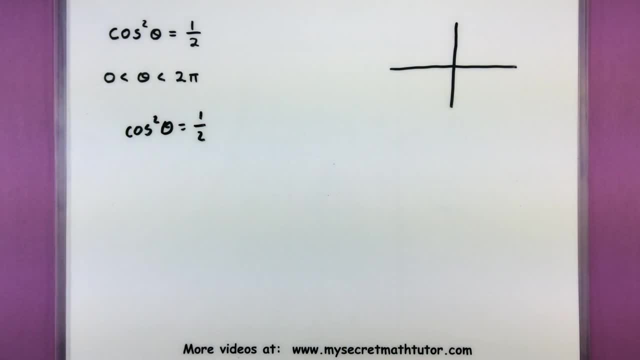 I'm really dealing with cosine squared, So before I can actually pick out key values on my unit circle, I want to get cosine all by itself. So we're going to take the square root of both sides. We're taking the square root of something squared. this will be plus. 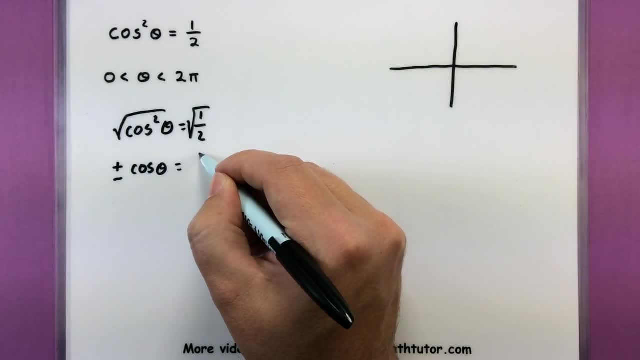 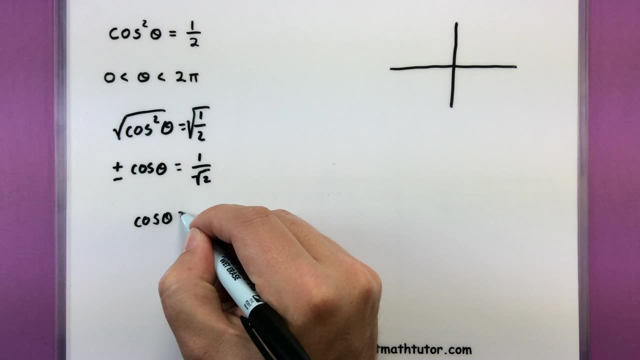 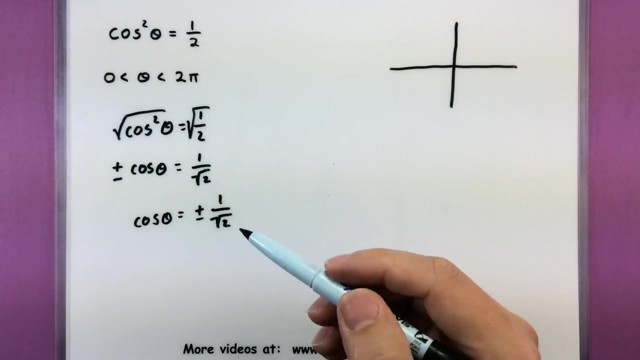 minus cosine of theta equals the square root of 1 all divided by the square root of 2.. Not bad, Let's go ahead and move the plus minus to the other side and it almost looks like one of our key values. Let's go ahead and multiply the top and. 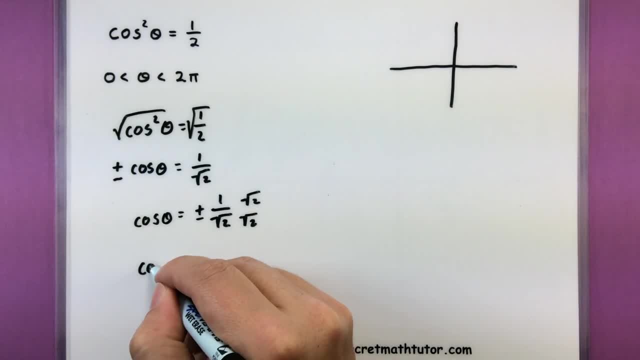 bottom by the square root of 2 and see that, sure enough it is We're looking for when cosine is equal to plus or minus the square root of 2 over 2.. All right, now we can turn our attention over to our unit circle and 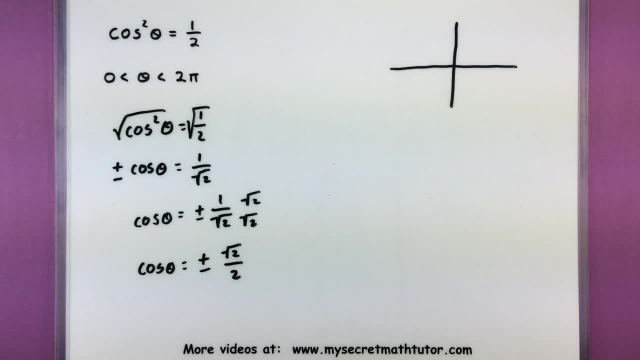 and now we're looking where every first coordinate is square root of 2 over 2, or whether it's a negative square root of 2 over 2.. So let's think of the values we'd get on there. So let's see, I have one angle up here that'd be square root of 2 over 2.. I have 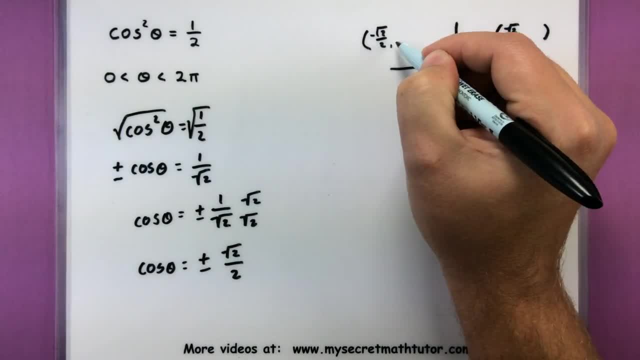 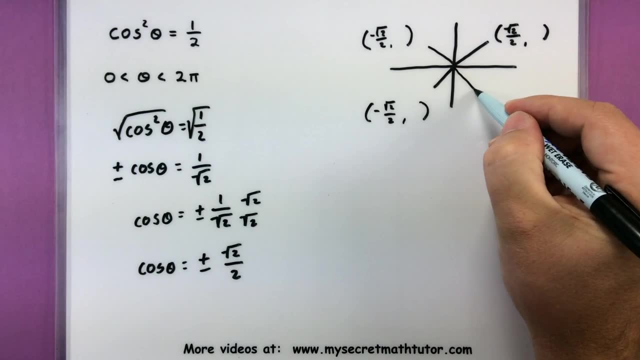 another angle over here, that'd be at negative square root of 2 over 2.. We have one down here, negative square root of 2 over 2.. And one more square root of 2 over 2.. Done, So what angles are these? Let's list. 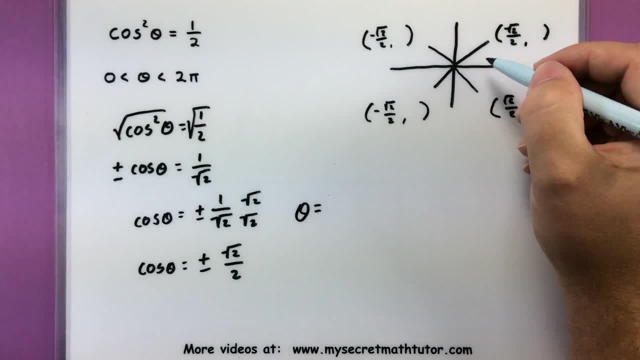 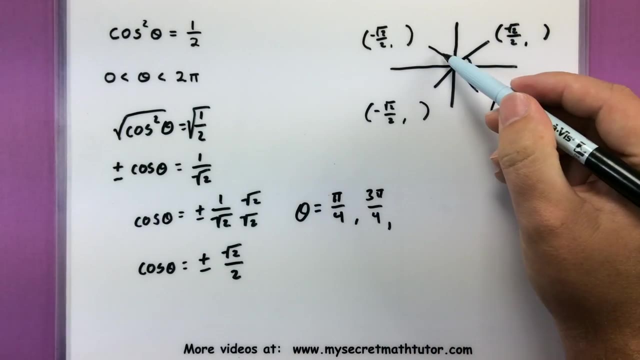 them all out so we can get all of the angles that satisfy our conditions. Well, the first one will happen at pi over 4.. Then we'll go and see 1, 4, 2, 4, 3, 4, so 3 pi over 4, to get the next one, 3, 4, 5, 5 pi over 4. for the next,